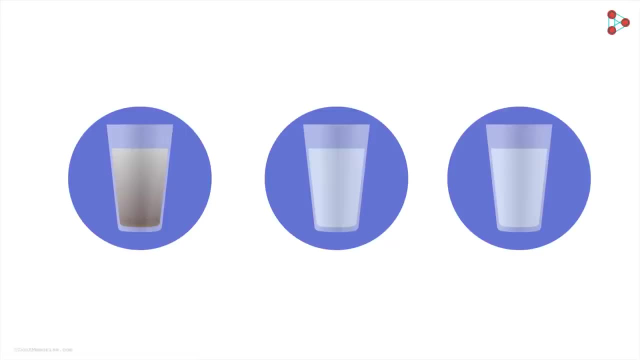 In one of them we've added mud, In the other we've added salt and in the third we've added sugar. Can you identify which glass has which mixture just by looking at them? Yes, I can, So let's take a look at them. 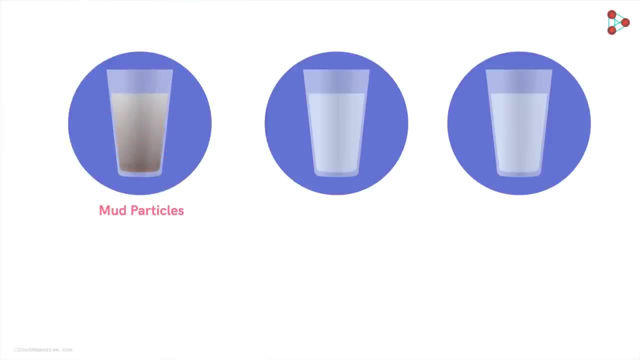 OK, You can easily identify the muddy water, but what about the other two? We can't differentiate between the other two as both the mixtures look just like water. This is because, in these two cases, we cannot see the dissolved salt or the sugar particles with our naked eyes. 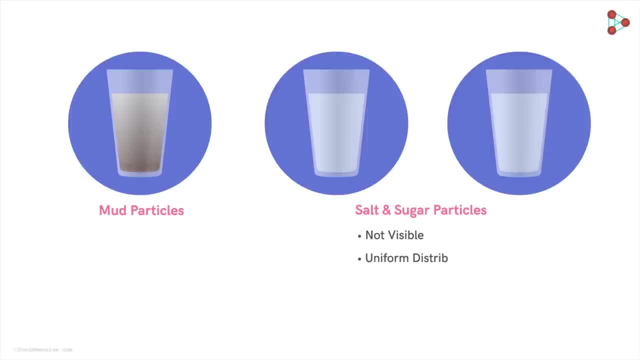 The salt and the sugar particles are evenly distributed in water, Whereas in the glass with the mud and water we are easily able to see the mud particles suspended and settled in the glass. So we can see that there are two types of mixtures. 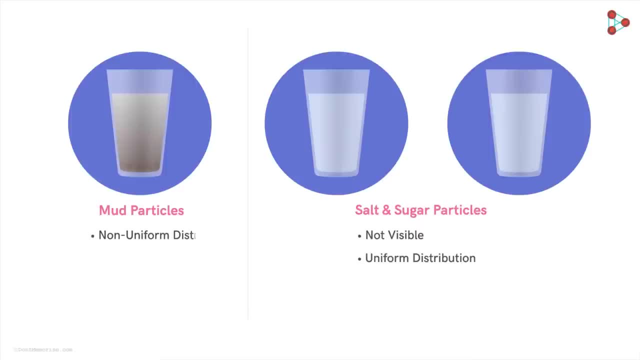 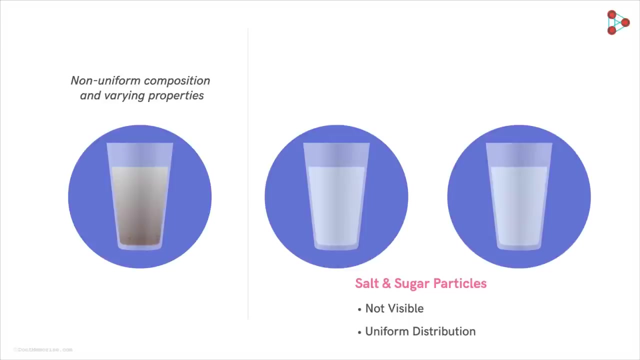 In the first mixture, its composition is not uniform and its components are in different phases, That is, you are able to see the different components separately. So this type of a mixture which has non-uniform composition and varying properties is called a heterogeneous mixture. 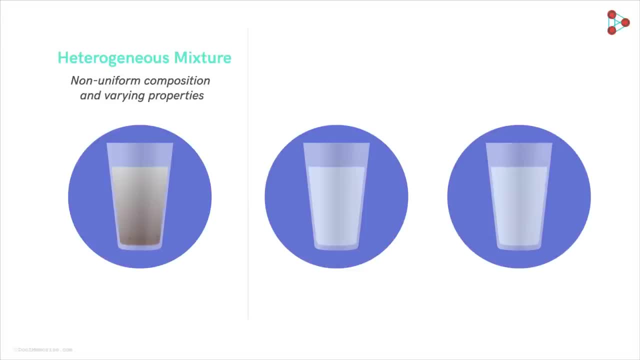 And in the second and the third mixtures. the mixture is not uniform mixtures. their composition is uniform throughout And its components are in a single phase, ie we cannot separately see the individual components. So this type of a mixture in which its composition 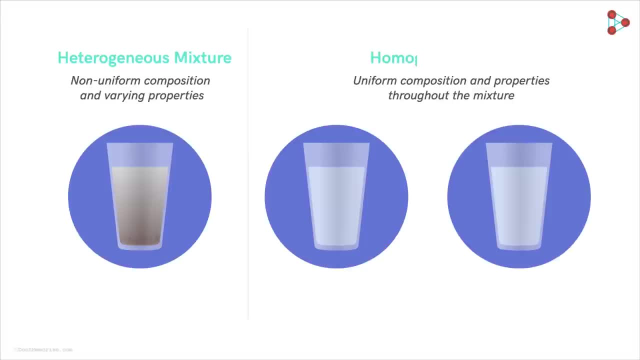 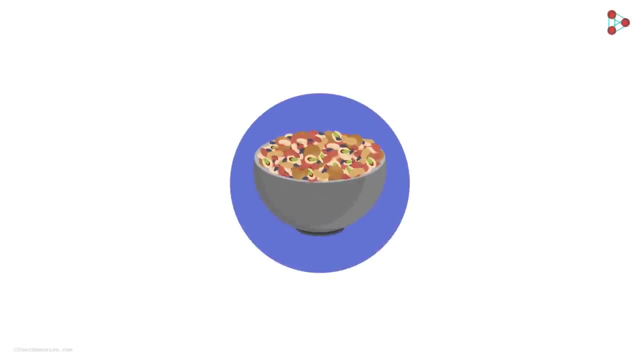 and properties are uniform throughout is called a homogeneous mixture. For example, in a bowl full of mixed nuts, it is possible to identify the different nuts in the bowl And the composition of the mixture is not uniform, So it is a heterogeneous mixture. Can you tell me if? 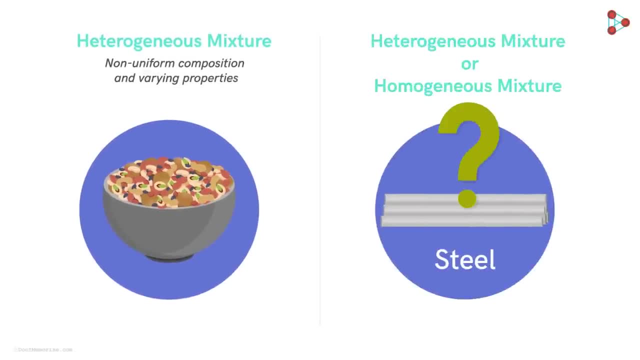 a block of steel is a heterogeneous or a homogeneous mixture. Steel is a mixture of mainly iron and carbon, along with some other elements, But these different components are not visible to our naked eyes And its composition looks uniform throughout the mixture, So it is a homogeneous mixture. Now, these types of homogeneous mixtures: 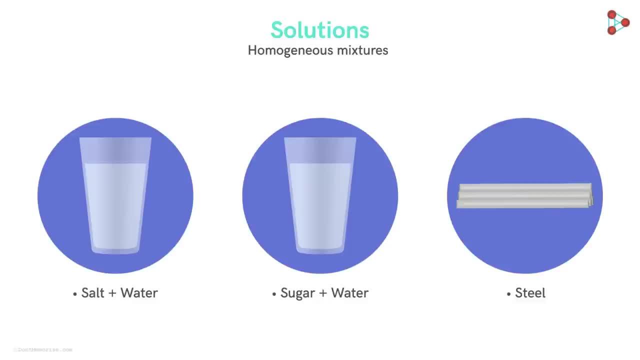 are called solutions. That is, a solution is a homogeneous mixture of two or more components. So here, the mixture of salt and water, the mixture of sugar and water and steel are all solutions. But wait, As we saw before, we usually think that solutions are always.